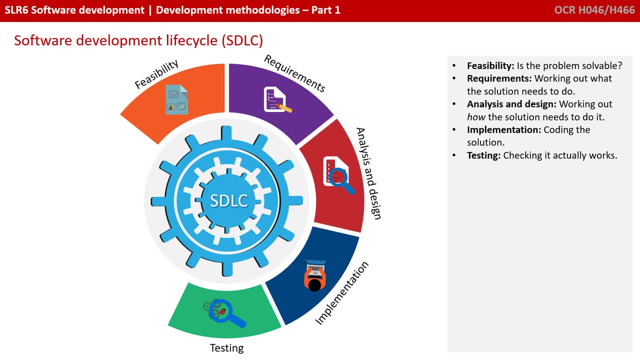 Obviously, having written any code, we have to test it thoroughly to check that it actually works. If it does, we can then deploy our finished solution, and this means installing it in the target environment. offenders: smaller because this is a local network network. You cannot have the software success in a private environment and I will not pick up years because you have to work on me, so work. 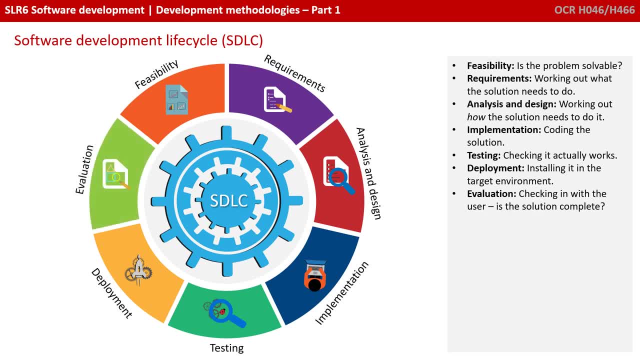 number five can be a good approach. If my problems work, I can pick it up and cut it apart later when I need Yong Darling. And of course we should always evaluate or review our program, Check it with the user. Is the system complete? Does it meet all their original needs and requirements? 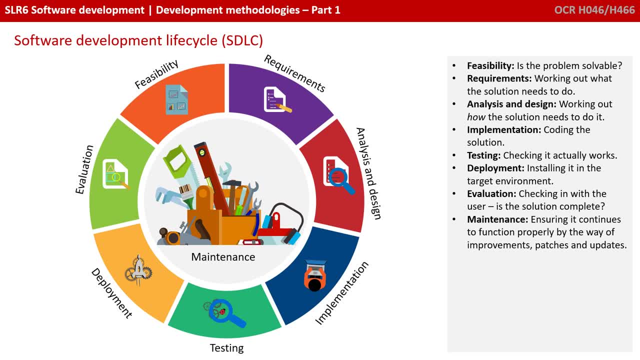 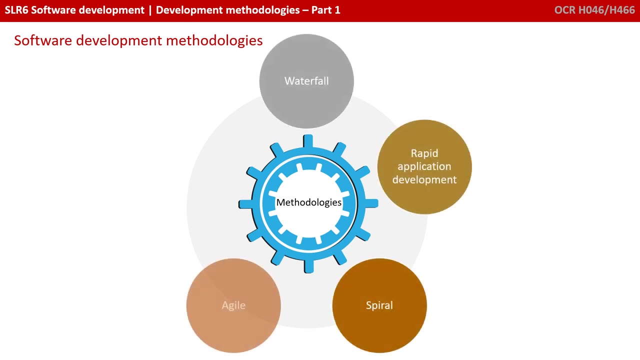 Often considered. another phase is maintenance. Now, this shouldn't be underestimated, and sometimes it's the longest phase of all the software development phases. This is where we make sure the software carries on working. We make improvements, patches, updates and additional releases. So I've mentioned there's five methodologies in specific that you're required to know about for the exam: Waterfall, Rapid Application Development, Spiral, Agile and Extreme Programming. 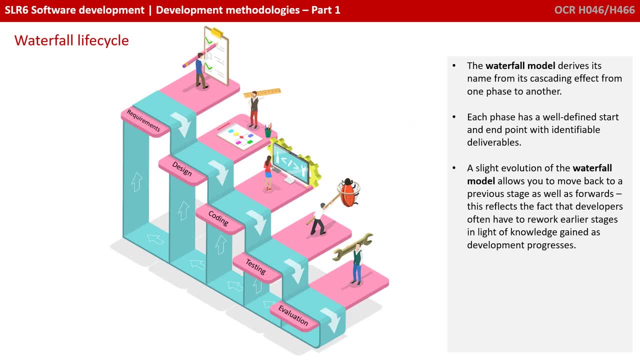 Let's take a look at them now. So what are they? So the waterfall model is one of the oldest and it derives its name from the cascading effect from one phase to another. Each phase has a well-defined start and end point with identifiable deliverables. 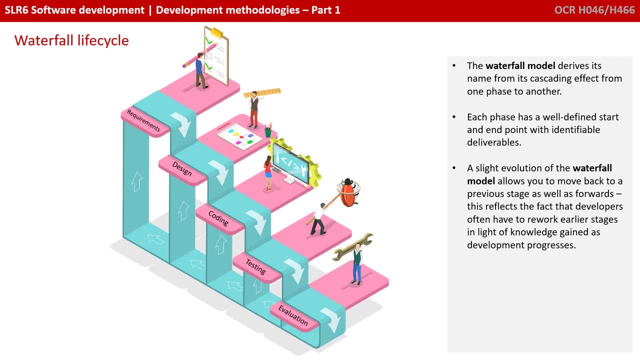 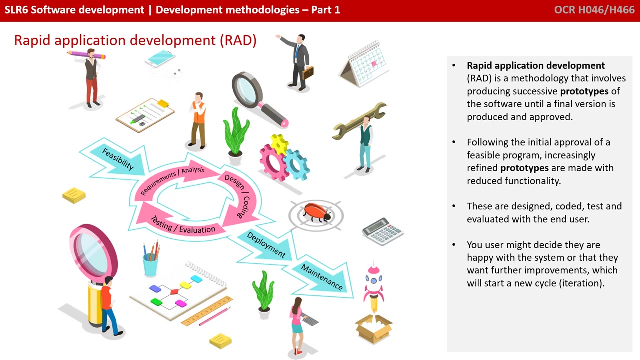 A slight evolution of the waterfall model allows you to move back to a previous stage as well as forwards, And this reflects the fact that developers often have to rework earlier stages of a project in light of experience gained as the development progresses. A much better evolution of the waterfall model is what's known as Rapid Application Development, or RAD. 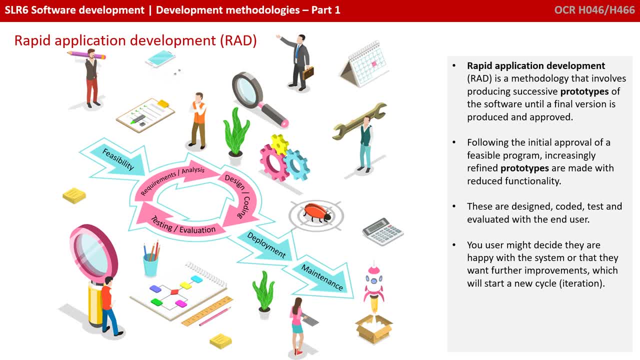 It's a development methodology that includes producing successive prototypes of the software until a final version has been produced. So, after the initial approval of a feasible program, we then enter a stage where we do some requirements, analysis, design, coding, testing and evaluation and produce a prototype. 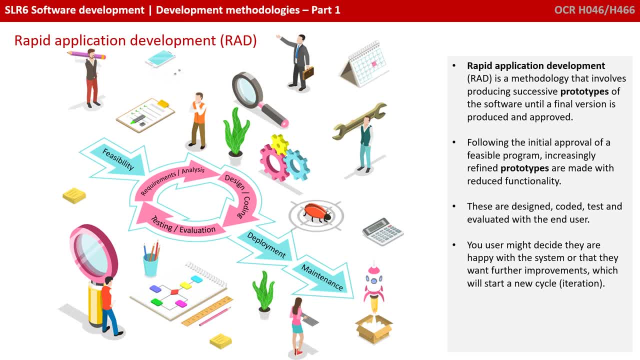 Each prototype is shown back to the user, who provides some feedback. These are designed, encoded, further evaluated. At any point during this cycle the user might decide they're happy with the system or might decide they want even further improvements or functionality, And of course this leads to a new requirement and the start of a new cycle or iteration. 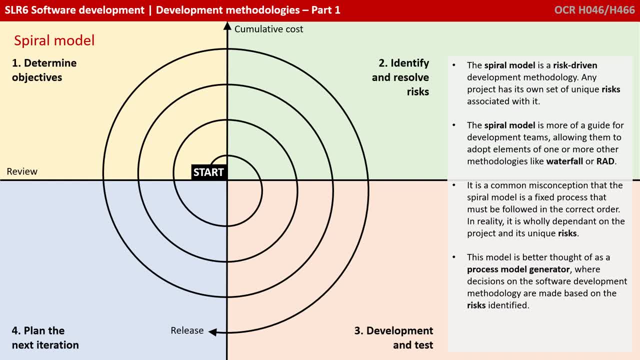 Next is the spiral model. Now, this is a model which is often really misunderstood. The most important thing to realise here is: the spiral model is a risk driven software development process model. Any project you embark on has its own set of unique risks associated with it. 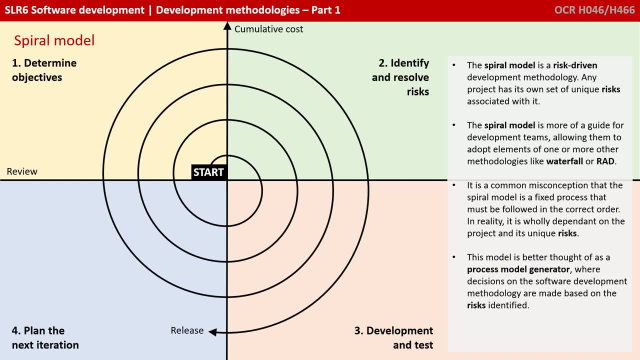 The spiral model, technically, is really more of a guide to development teams. It allows them to adopt elements of one or more other methodologies, such as waterfall, RAD, agile, etc. It's a common misconception that the spiral model is a fixed process model and that every activity we're about to show you must be followed in the order given. 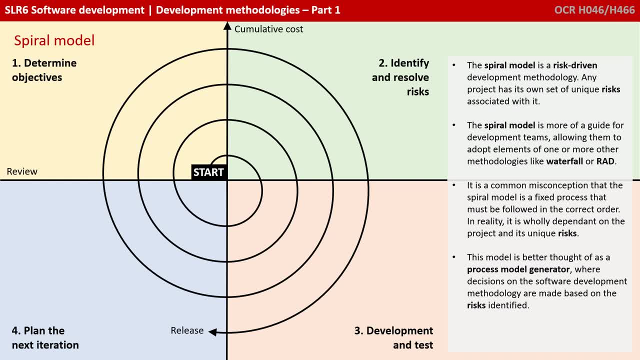 It is wholly dependent on the project and its unique set of risks. This methodology is really better thought of as a process model generator, Where choices on the actual software development methodology are chosen based on the risk identified. It's split into four main quadrants. 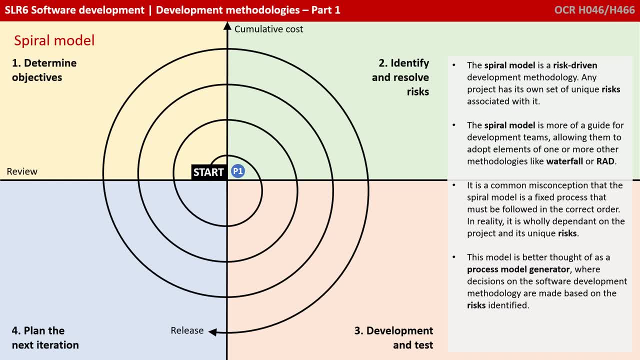 Determine the objectives, Identify and resolve risks, Develop and test And then, if necessary, plan for the next iteration. You can see here we've started in the top left, determining some objectives and that may lead to a very early initial prototype, prototype one: 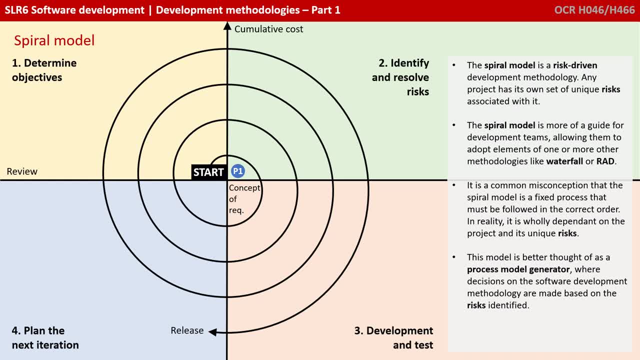 From this we can build an initial concept of requirements, We can build a concept of how this system will operate, And we can develop a very initial prototype, We can develop a very initial requirements plan. It's at this very first stage that we would then commit to an appropriate methodology for the next iteration. 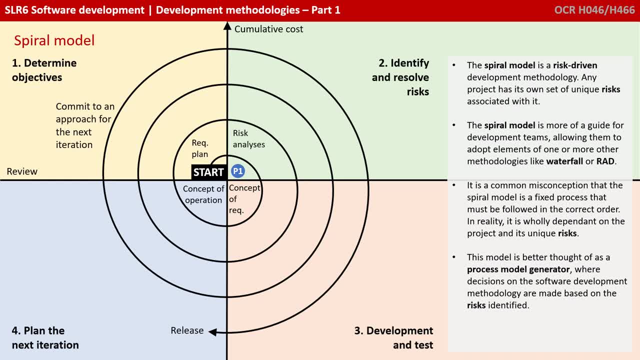 At this point we would carry out a risk analysis. What are the risks of this current system? How do we overcome them? A second prototype can be developed which can be shown to the user. Out of that will come some more requirements. 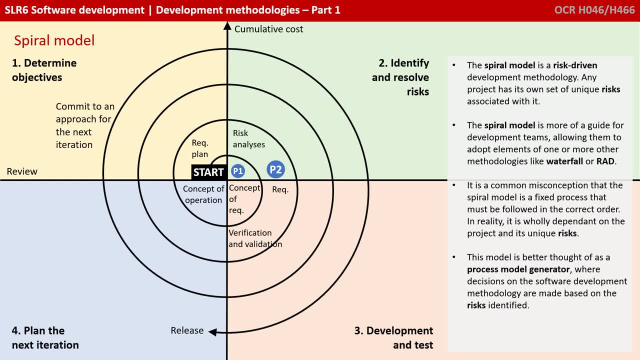 We would verify and validate the second prototype and the second set of requirements, And we would produce a development plan. At this point, our system is starting to take more shape. We then need to commit to an appropriate approach for the next iteration, Where again, we analyse any risks that have arisen. 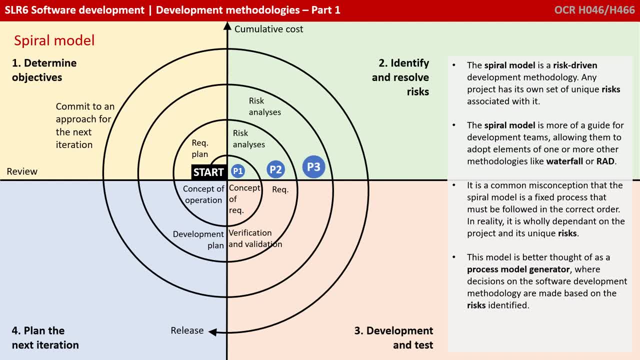 Each time round we're producing a successive prototype, much like the RAD model, And hopefully the risks are decreasing and the user and the development team are becoming more comfortable with how the product is proceeding. We would verify and validate everything we've done. 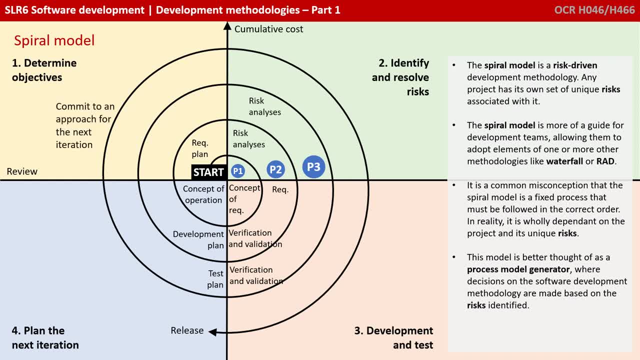 Possibly at this stage, come up with a test plan And commit to an approach for the next iteration, But always taking in mind any risks which were arising Now. at this point, our spiral model has effectively finished and we're coming up with what we're calling an operational prototype. 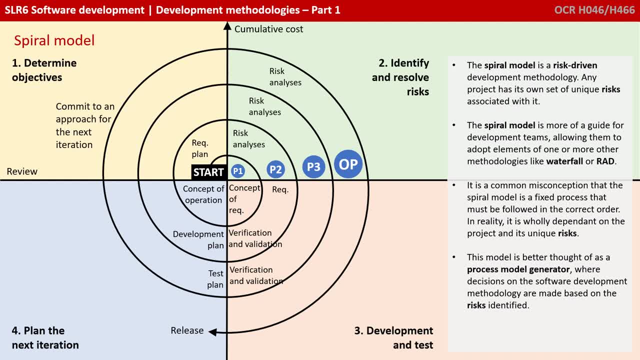 But, as mentioned, you may go round this spiral two times, four or six- It's not necessarily fixed or in this order. The point is: by focusing with risk at its heart, you should eventually achieve an operational prototype Which is most appropriate for the user. 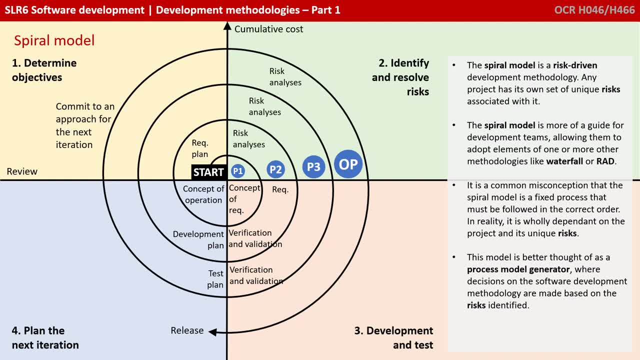 And has been developed up to that point using the most appropriate development methodologies. It's only at this stage where we actually enter the main part of development and testing. We now have a detailed operational prototype. We can do a proper design code unit test to integrate it. 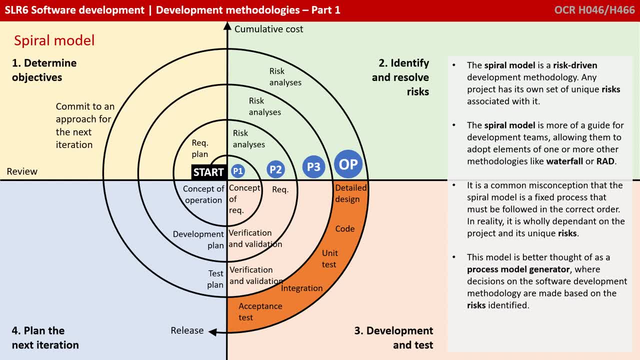 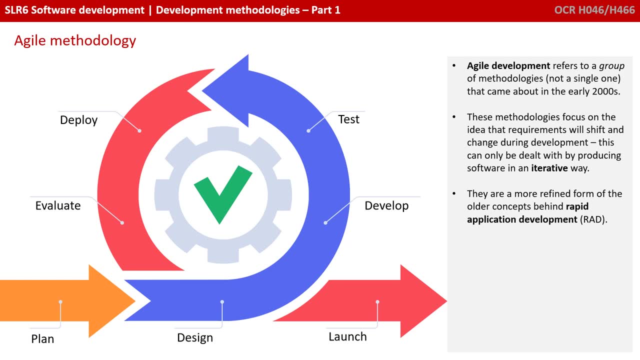 Make sure we get it accepted by the user And then finally release it. Although this model looks quite complex, the important thing to remember here for the exam is the spiral model is a risk driven development process. Now let's turn our attention to agile methodologies. 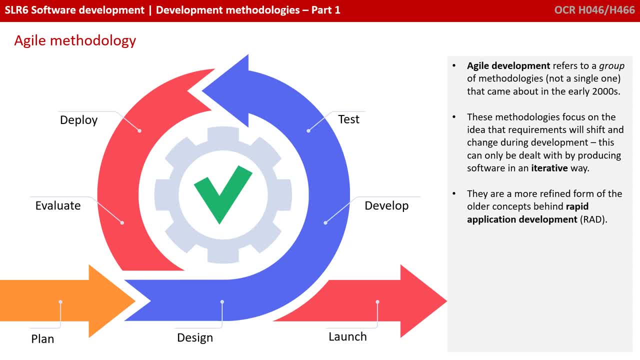 So agile development actually refers to a group of methodologies and not technically a single one, And they started to become popular in the early 2000s. These methodologies focused on the idea that the requirements will shift and change during development And this can only be dealt with by producing and developing software in an iterative way. 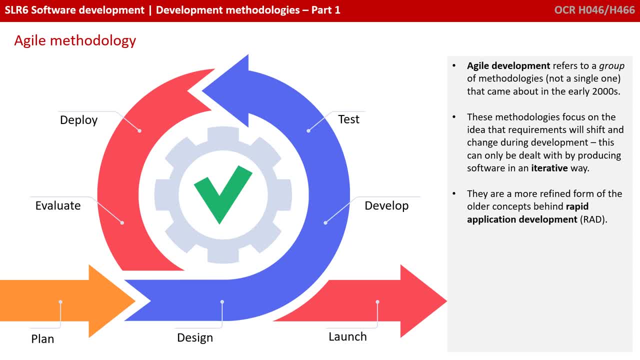 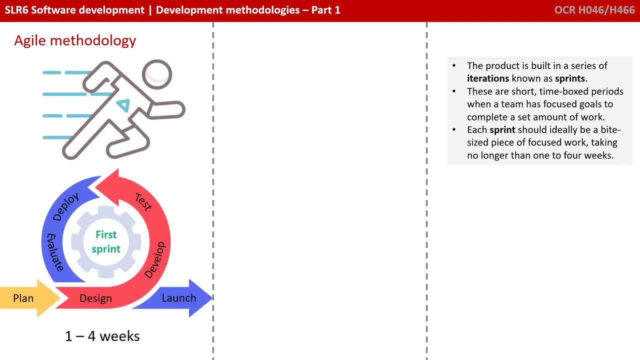 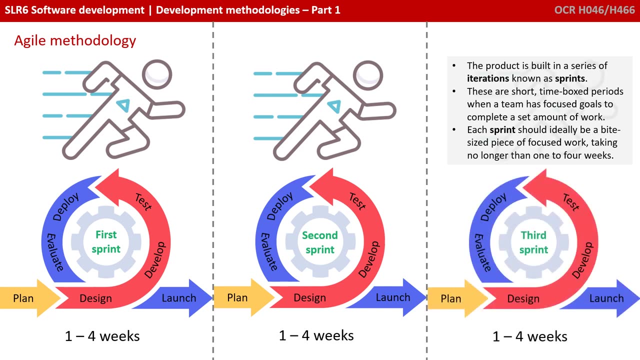 They're a more refined form of the older concepts behind rapid application development. At the core of agile methodologies is the idea of building each iteration in what is known as a sprint cycle. Sprints are short time boxed periods when a team has focused goals to complete a set amount of work. 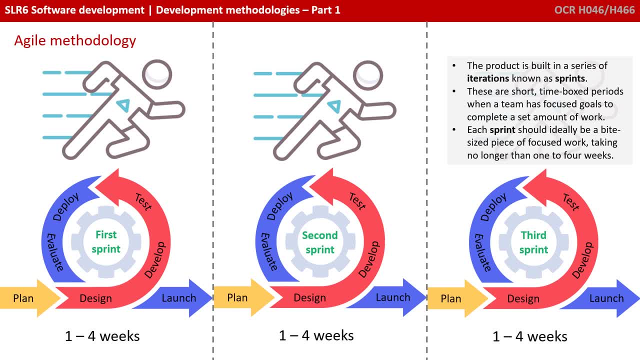 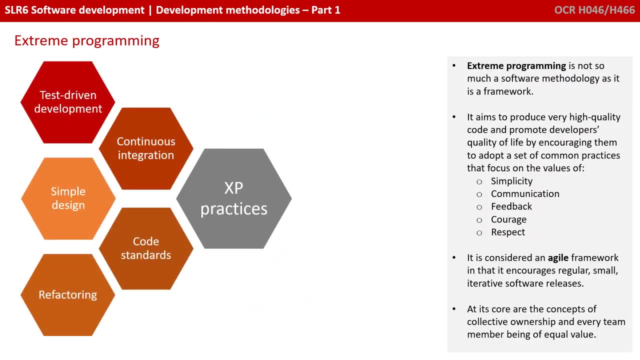 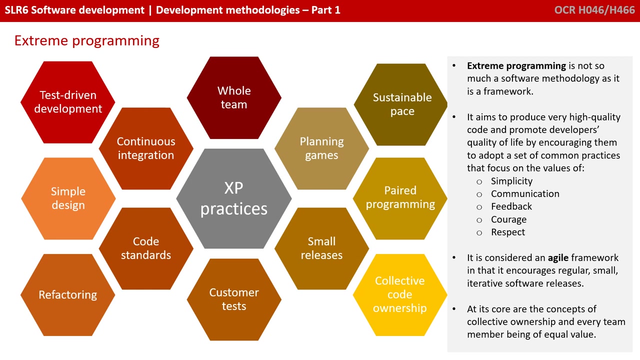 A very important concept of agile methodologies is the idea that each sprint should ideally be a bite sized piece of focus work, typically taking no more than one to four weeks maximum. Finally, let's talk about extreme programming. So this is again not so much a software methodology as it is really a framework. 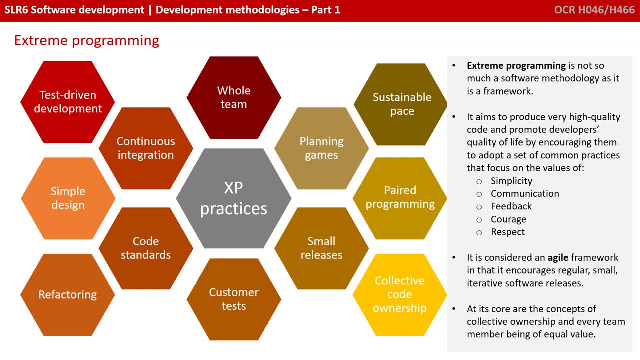 Extreme programming aims to produce very high quality code and promote developers quality of life by encouraging the team to adopt a set of common practices that focus on simple values like communication, courage, feedback, respect and simplicity. It is itself considered an agile framework and that it encourages regular small iterative software releases. 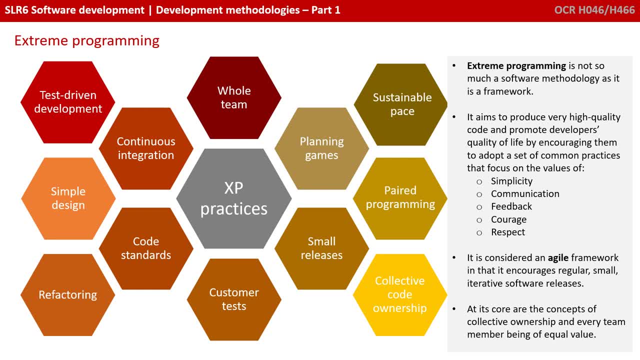 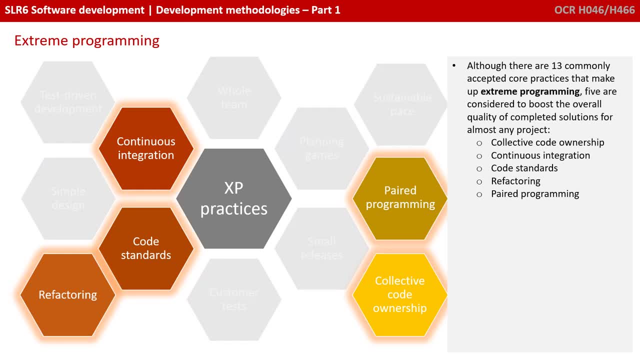 At its core are the concepts of collected ownership and every team member being of equal value. Now there are technically 13 commonly accepted core practices that make up extreme programming, And these aren't listed in the specification, so you don't really need to understand what each of these are. 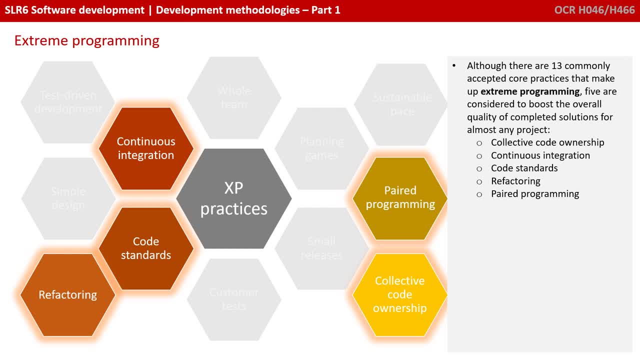 But there are five which are considered on average to boost the overall quality of the completed solution of almost any project. There's the idea of collective code ownership, that everybody is in charge of the entire code base. The idea of continuous integration, high code standards, refactoring, which means revisiting old code. 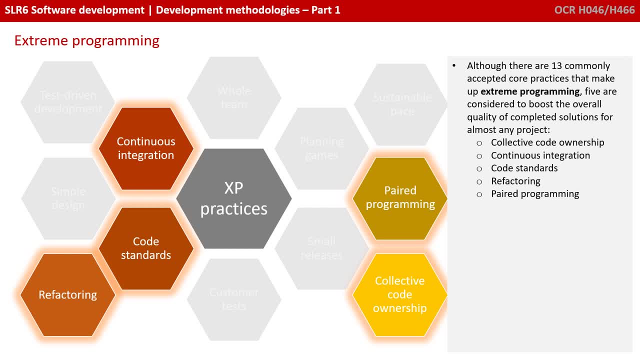 and repurposing it to make it more efficient and more robust, And an idea of paired programming. This is literally the idea of having two programmers sat side by side at the same computer screen and keyboard. It's the idea that two sets of eyes are better than one and that higher quality code will end up being produced.